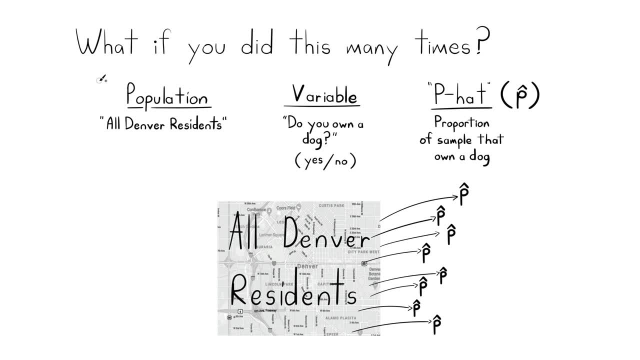 And then imagine what if we took a lot of samples from the same population with the same variable. So each one of these arrows is representing the idea of collecting 40 people and finding out what proportion of them owns a dog, Taking many samples and finding many p-hats. 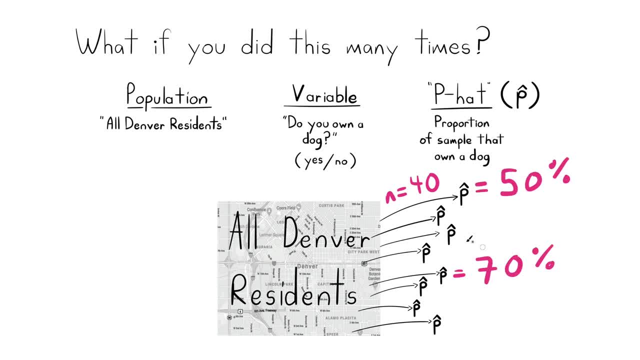 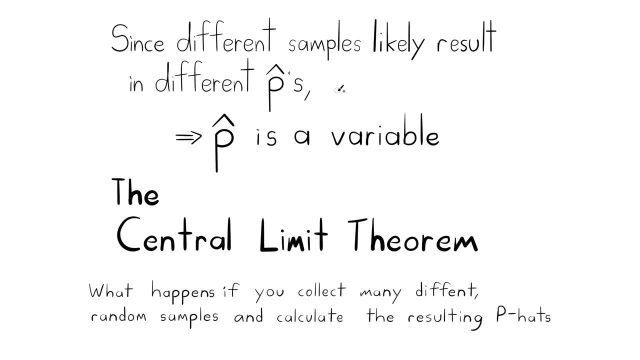 And you can imagine that we wouldn't get the same value every time. We're going to get different sample proportions And since different samples give us different p-hats, we can consider p-hat a variable. P-hat varies- It's not always the same- just like the color of a car varies or the height of a person is a variable. 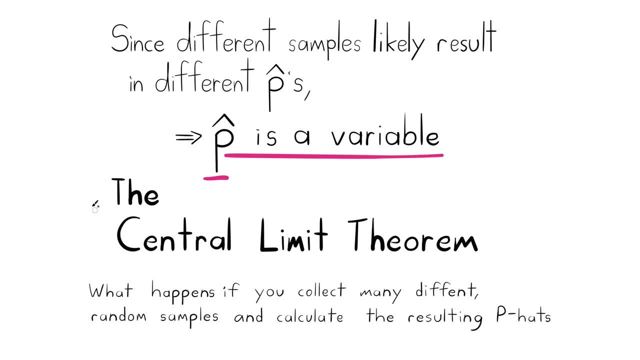 Our sample proportion is also different. It's not always the same, just like the color of a car varies or the height of a person is a variable, And there is a very important idea in statistics called the central limit theorem That's going to give us important information about what happens if you collected a lot of different random samples. 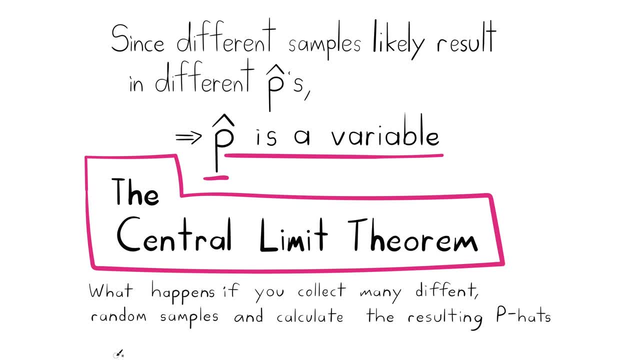 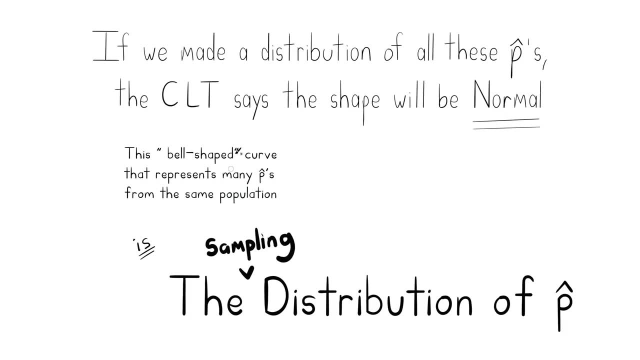 and found the sample proportion for each one of those. It's called central limit theorem because it is central to the subject of statistics. So first of all, if we made a distribution of all these p-hats, basically collected them all, and looked at if we saw any patterns, the central limit theorem says: 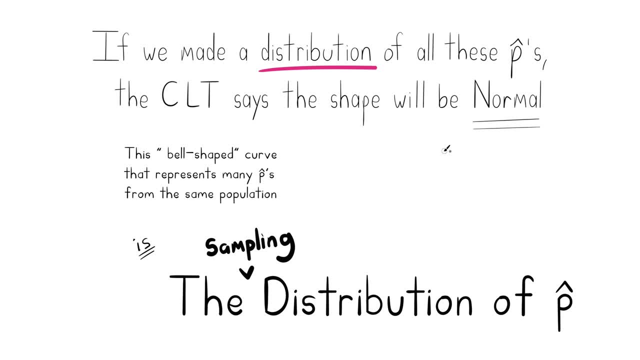 that the shape of this distribution will be normal, Normal meaning Gaussian, bell-shaped. and this bell-shaped curve that represents a lot of different p-hats from the same population is what this video is all about: the sampling distribution of p-hat, And sometimes the word sampling can be. 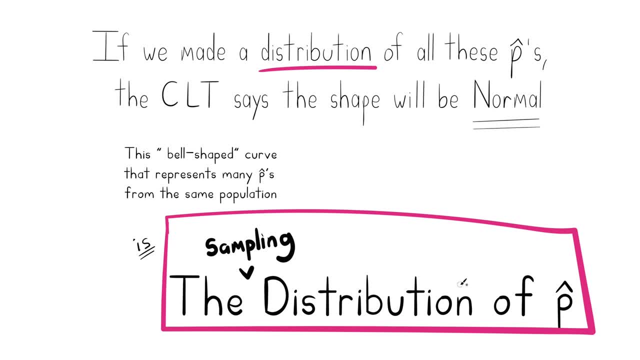 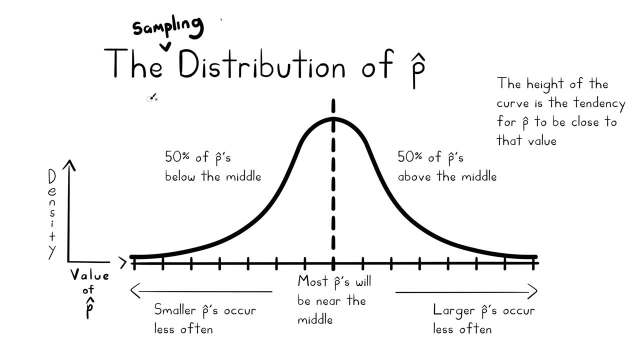 a little bit confusing, so I might just call it the distribution of p-hat. Either way, I'm referring to the same thing And this is what the central limit theorem tells us- what the pattern we would see. We would get this bell-shaped curve, where the height of the curve more or less represents: 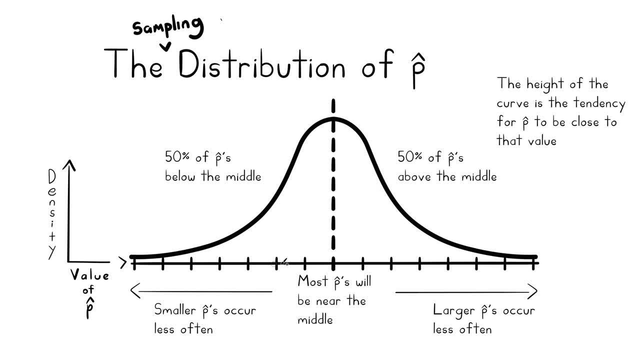 the tendency that p-hat will be a certain value. So right here in the middle is the most likely values of p-hat, and the higher the values of p-hat, the higher the distribution of p-hat, The less likely. and also, the lower the values of p-hat, the less likely. And that's true about. 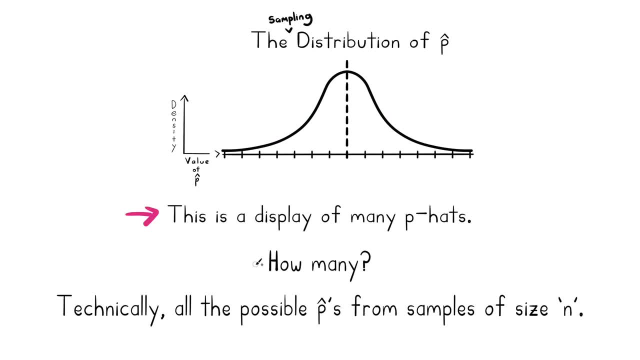 any variable that has a normal distribution. And just to get slightly more specific about what this thing means, how many samples is the distribution of p-hat referring to? Well, it's referring to all the possible p-hats you could take from a given population And typically, 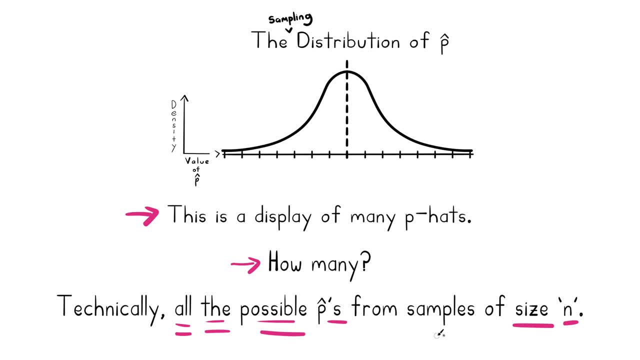 that's a lot if you think about. if you were sampling 40 Denver residents, there's maybe a million Denver residents, and the amount of groups of 40 of them you could have is quite a few. And so when you're actually conducting statistics, 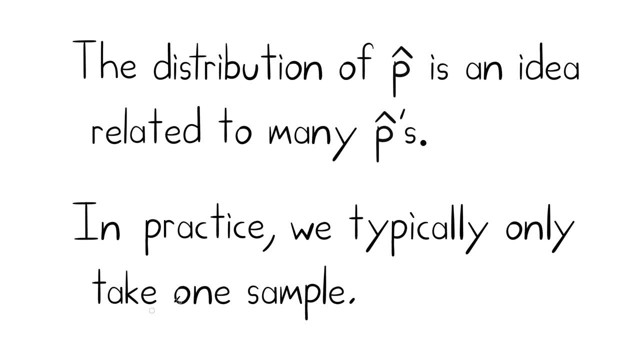 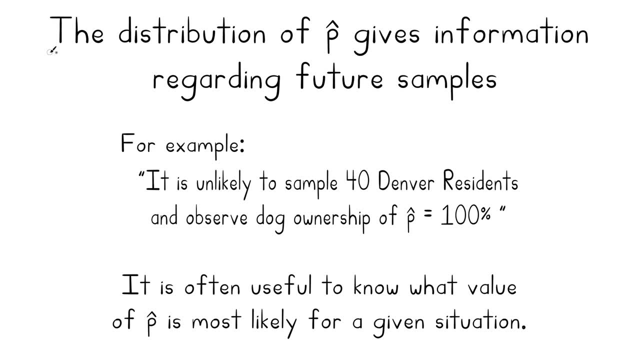 you don't go out there and take a lot of different samples. In practice we usually only take one sample. say something like this: because of the central limit theorem and the distribution of p-hat, It is unlikely to sample 40 Denver residents and observe. 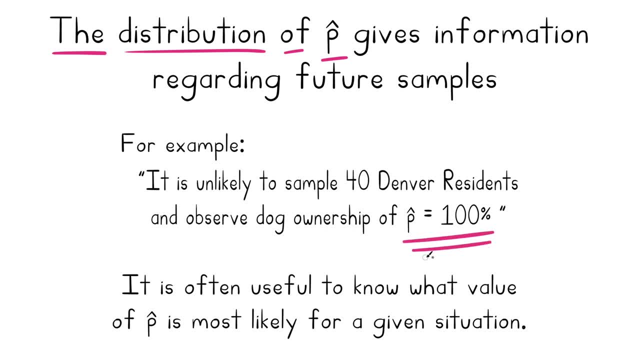 dog ownership of p-hat. P-hat equals 100% Because of the central limit theorem, a statement like this is true, Although you could kind of say, hey, I didn't need to know the central limit theorem to know that it's unlikely that everybody I sample will own a dog, And I think that's a nice thing about. 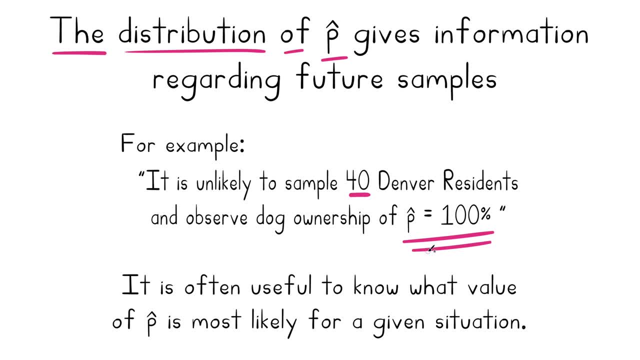 this whole idea is that some of the important concepts are somewhat intuitive- And I think that's a nice thing about statistics in general- And so a value of a hundred percent for p-hat would be unlikely, But it's often useful to know what value of p-hat is most. 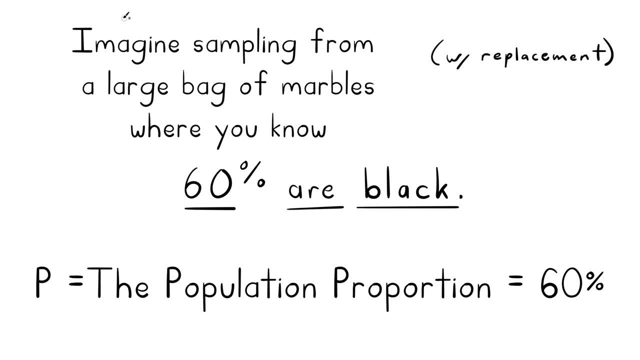 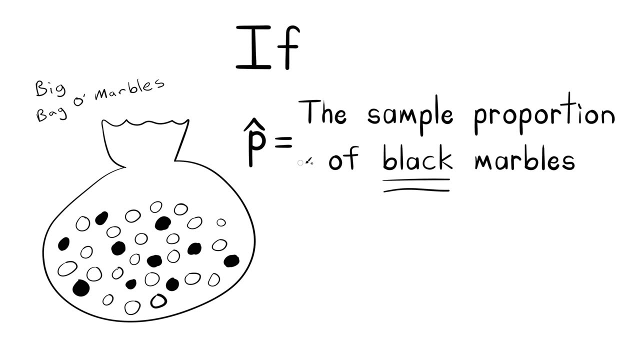 likely To explore the idea of the most likely value. imagine sampling from a large bag of marbles where you know that 60% of all the marbles are black. That's capital. P is 60%. So if we were sampling from that bag of marbles and finding the sample proportion of black, 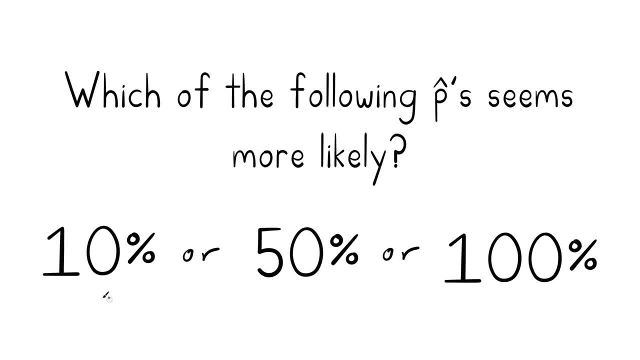 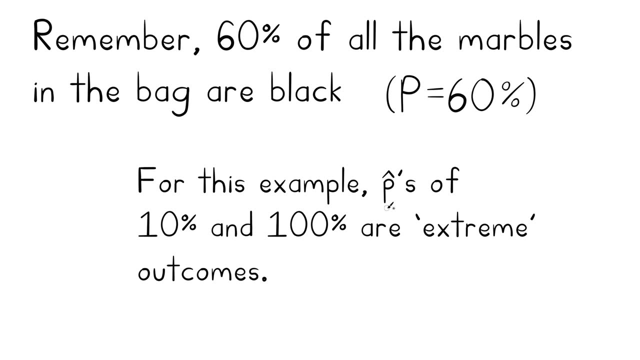 marbles. which of the following p-hats seems more likely: 10% or 50% or 100%? Remember that 60% of all the marbles in the bag are black And because of that, a sample proportion of 10% or 100% are what we could refer to as extreme outcomes. They're somewhat unusual. 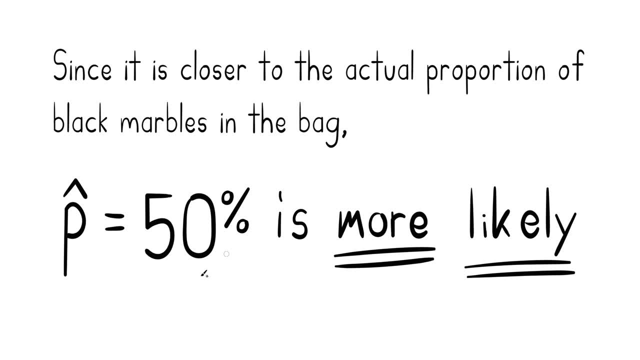 Since it is closer to the actual proportion of black and white, we could say that the of black marbles in the bag, a sample proportion of 50%, is more likely. The values of 10% and 100% are further from the true population proportion of 60%. 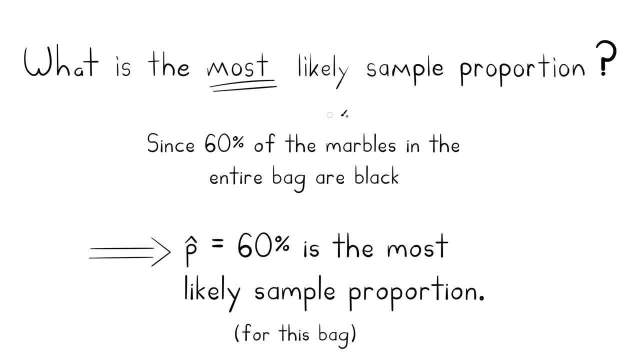 What is the most likely sample proportion, and this is a really intuitive result, I think. since 60% of all the marbles in the bag are black, a sample proportion of 60% is the single most likely sample proportion to observe. It's certainly not guaranteed, but if you had to bet on what value of the sample? 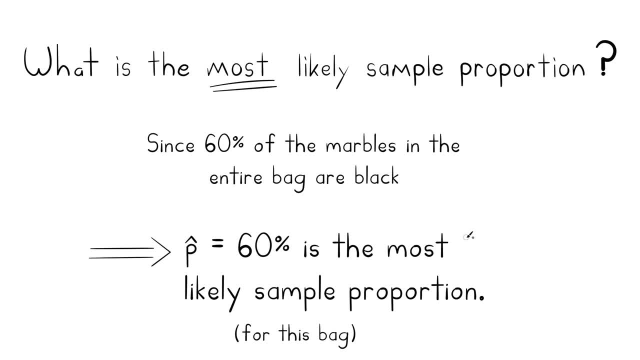 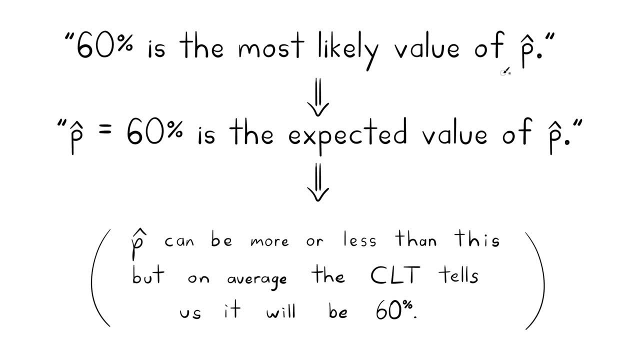 proportion, you would see 60% would be the number you should put your money on. So we could say 60% is the most likely value of p-hat for this bag of marbles. 60% is the expected value of p-hat On average. the central limit theorem tells us that we'll get 60% and 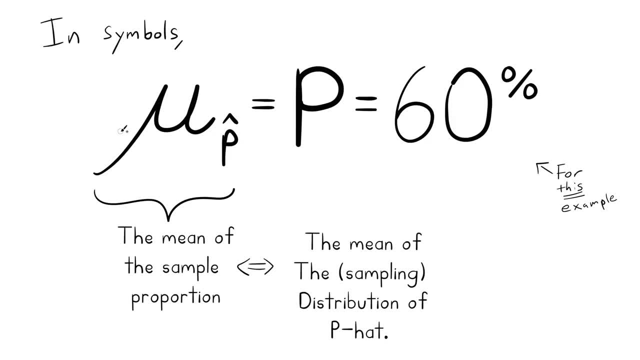 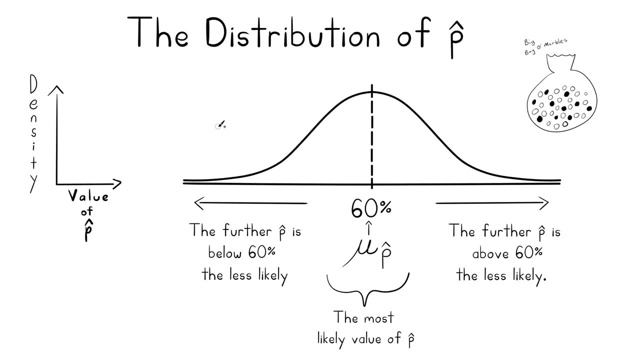 what this looks like in symbols. we're gonna call the average value of p-hat, mu with a subscript p-hat on it, and that equals whatever the population proportion is. And so what that looks like if we put it together with our normal distribution. 60% would be that number that's right in the middle, and 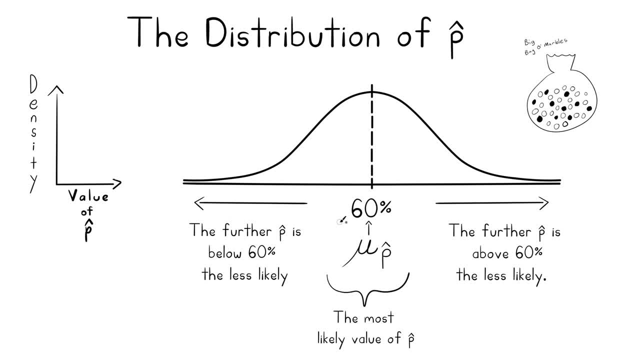 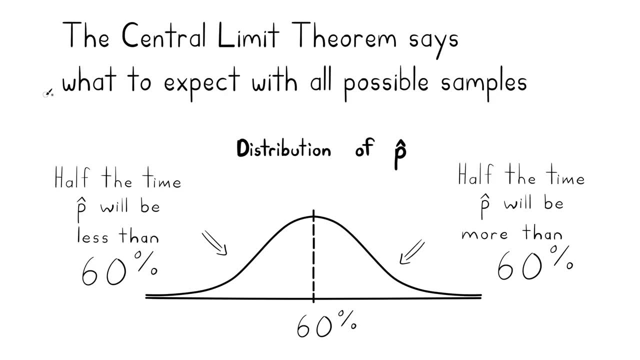 if we put it further with sample proportions above or below 60%, the less likely those values will be. We could say things like half the time p-hat will be more than 60% for this bag of marbles. We could say the probability of getting a. 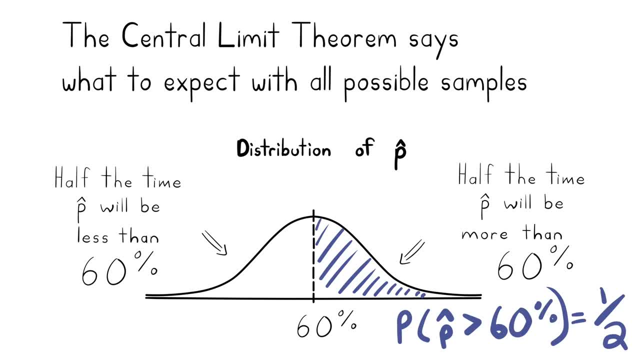 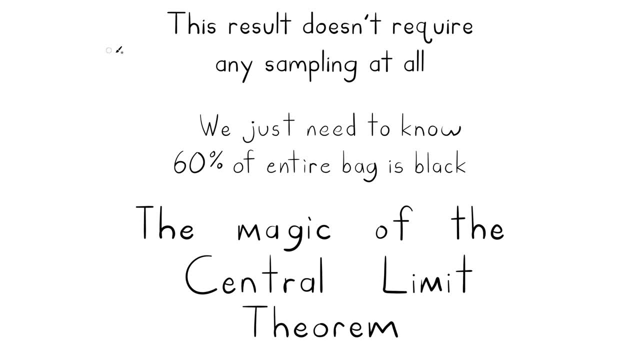 p-hat more than 60% is one half, And what's really nice about the central limit theorem is that it allows us to talk about all possible values of p-hat. We could say that if we put 60% of the entire bag of marbles in a sample, we 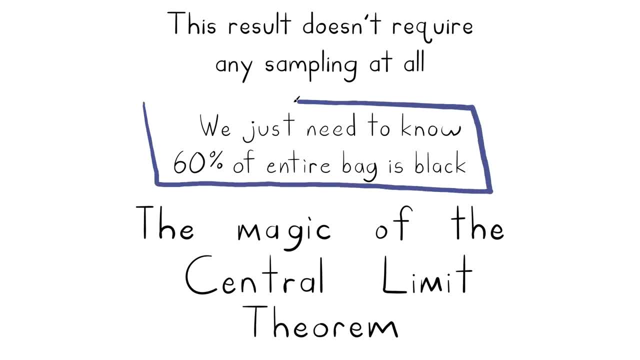 know that in the future the probability this proportion of black marbles in that sample will be more than 60% is one half, And we didn't have to even do any sampling. we just needed to know what was going on with the bag And that's kind of. 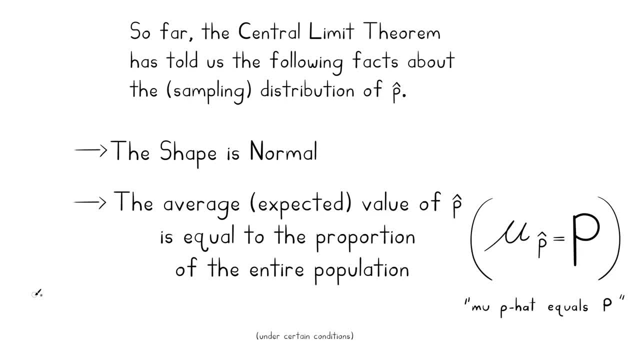 a beautiful result. So so far, the central limit theorem has told us the following facts about the central limit theorem: We know that the sampling distribution of p-hat, we know that the shape is normal, and then we also know that the middle of that distribution the expected value is equal. 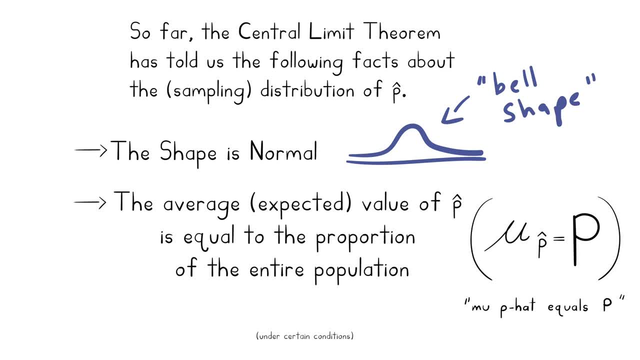 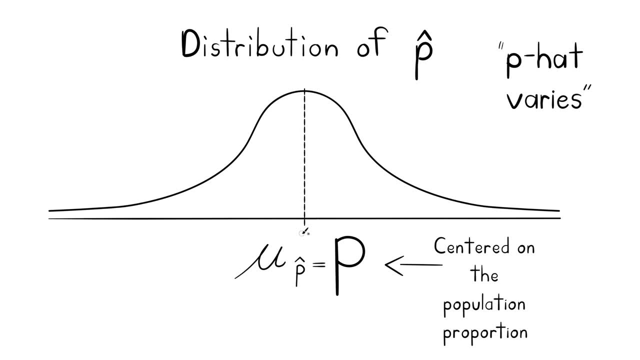 to the proportion of the entire population, And so what this looks like in a slightly nicer picture is the population proportion is right in the middle of the sampling distribution of p-hat. p-hat is a variable, and so let's do an example. problem related to the sampling: 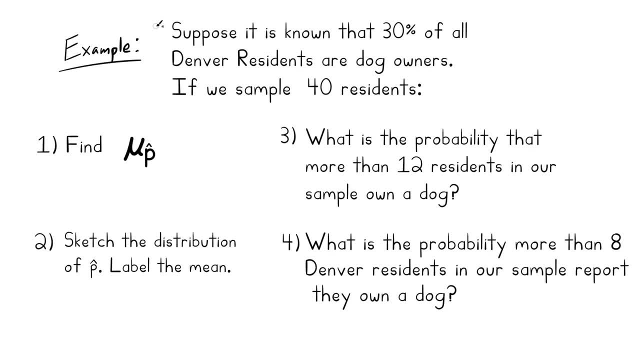 distribution of p-hat Suppose. it is known that 30% of all Denver residents are dog owners. If we sample 40 residents, here's a few problems we're going to be looking at. If you want to try to do these on your own right now, that might be a good idea From what you've seen in this. 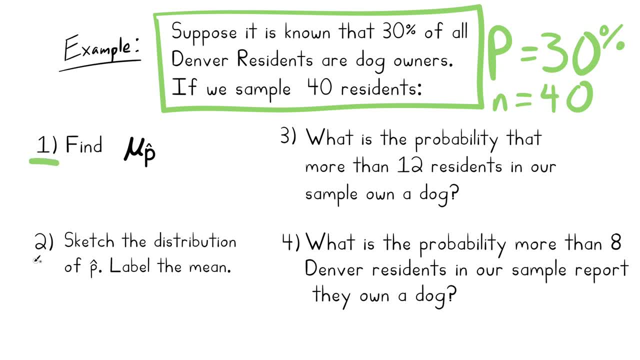 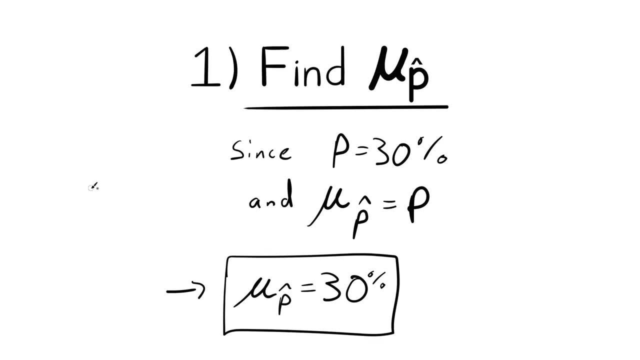 video. you should be able to do the first three problems, So let's get started on answering these questions. The first one is the easiest: Find the mean of the sampling distribution of p-hat. Well, since the mean of p-hat is equal to the population. 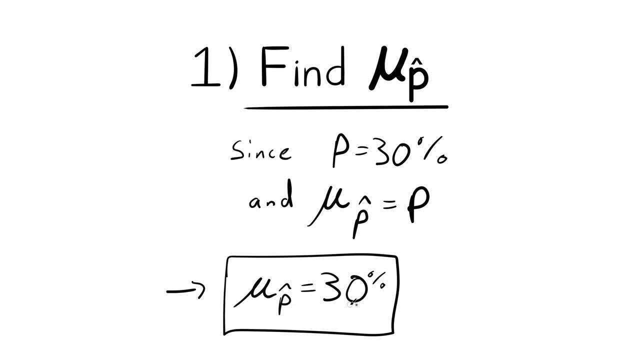 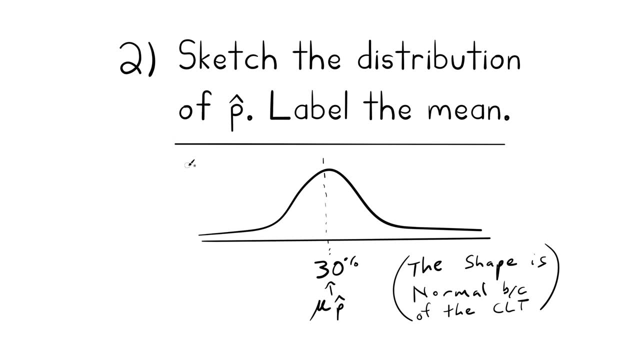 proportion, then that means that mu of p-hat equals 30%. And the second question reminds us what that is. If we're told to sketch the distribution of p-hat, well, that's a bell shaped curve. It doesn't look super nice in my picture, but it's just a sketch. And in 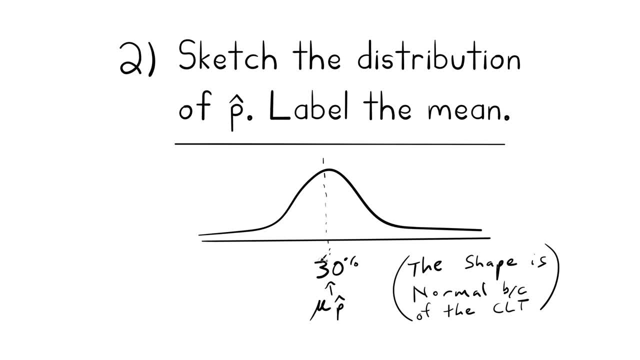 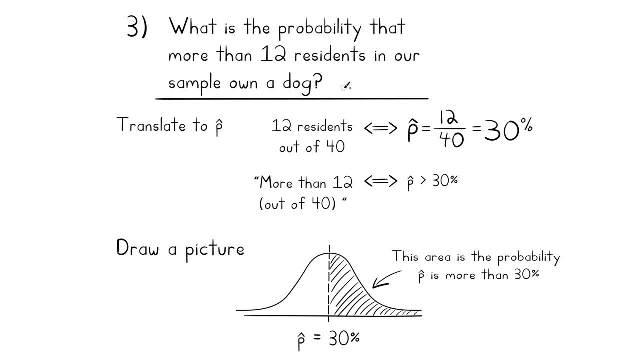 the middle of that curve comes the mean of 30%. Now we're asked: what is the probability that more than 12 residents in our sample own a dog? And that's a question about a count related to our sample And what we want to. 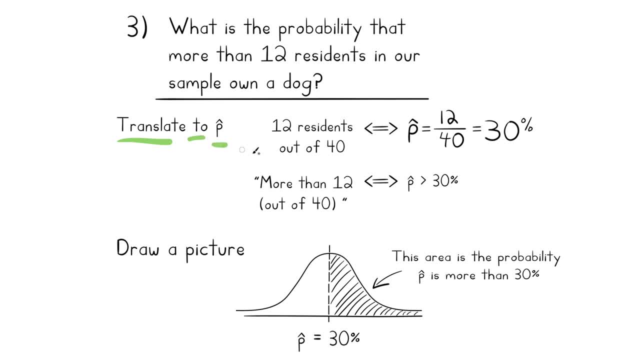 do is take that count and translate it into a proportion. 12 residents out of 40 means that p-hat would be 12 over 40, which would be 30%. If we're looking for more than 12, that means p-hat being more than 30.. 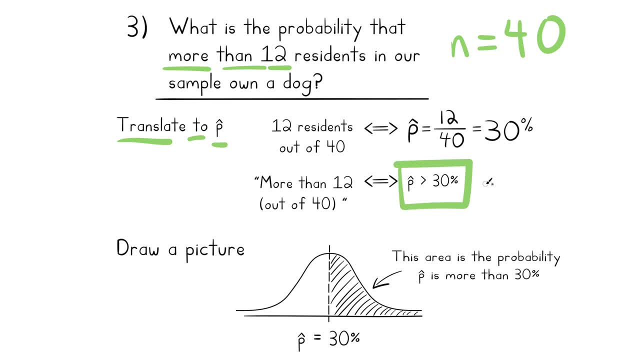 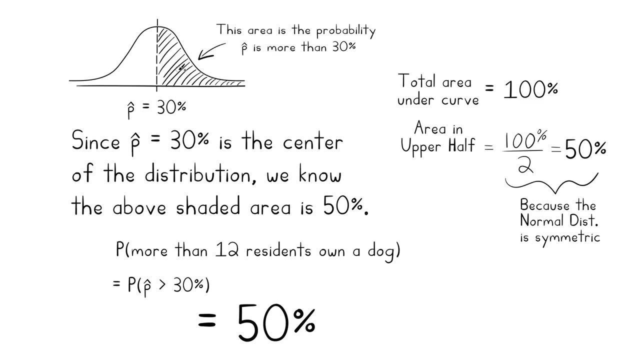 Where you just needed to translate that into a proportion, And I always recommend drawing a picture as well, taking a second to make a little sketch and shade in the area that you're trying to find. So we're trying to find this area here And we got a little lucky with this question. 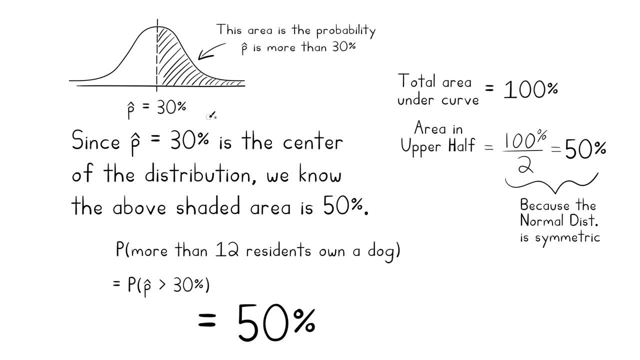 because 30% is the exact middle of this distribution And we're trying to find the area to the right of the exact middle, 50%. no formulas or calculators needed: percent, And sometimes it can be a little confusing because the variable that we're working with 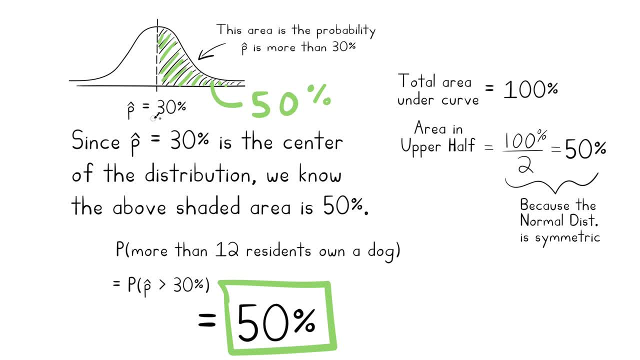 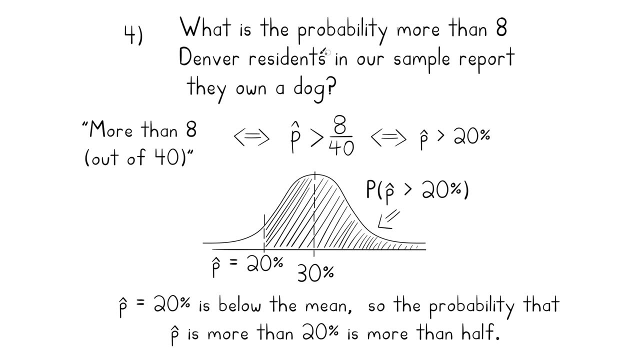 is a proportion which a lot of times we will talk about as a percentage, but also the answer is typically given as a percentage as well. So let's keep going. What is the probability? more than 8 residents in our sample report. they own a dog. 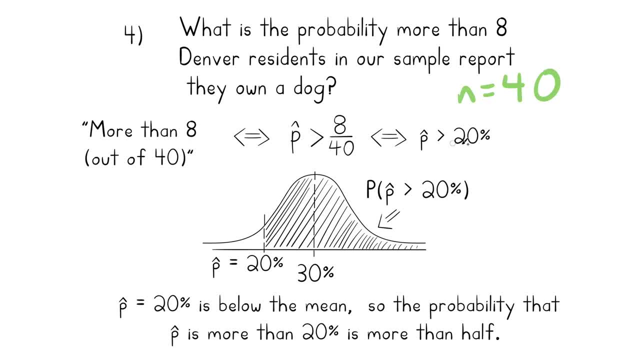 More than 8 is p-hat, more than 8 out of 40, which is a sample proportion now of more than 20%. 30% was right in the middle, which means that 20% is to the left of the middle. 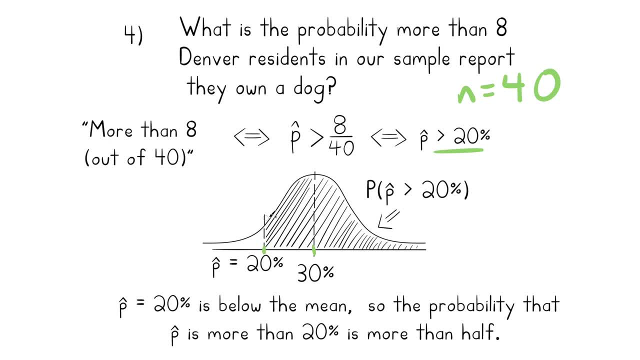 And so that means that the area to the right of 20% is going to be more than a half, And right now we don't actually have the tools- The tools that we need to answer this question. we know that it's more than a half, but there's. 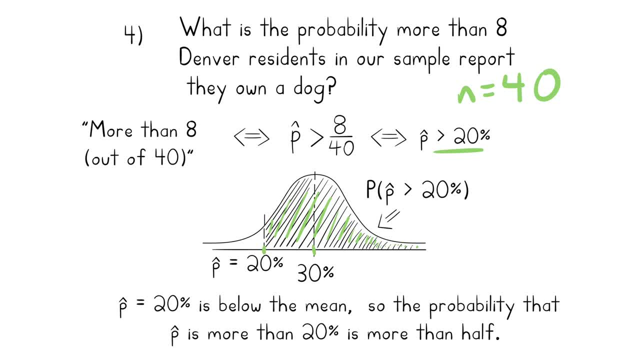 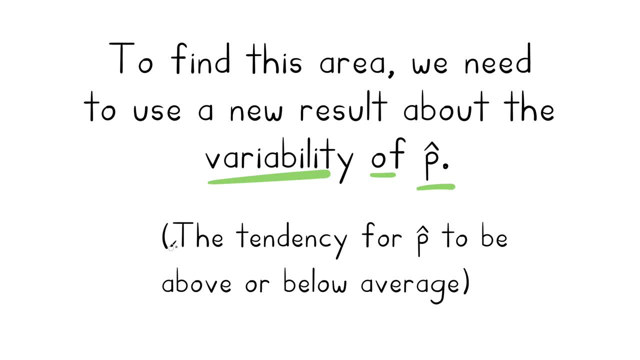 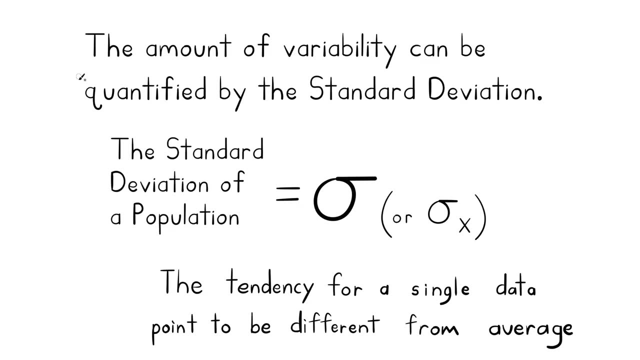 something else that we need to bring in to this problem now, And what we need is the variability of p-hat. How much tendency is there for p-hat to be above or below average? As a reminder, if we're talking about a quantitative variable in statistics and we want a number, 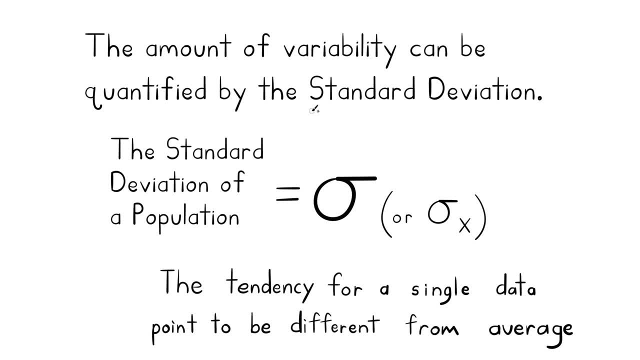 that tells us How variable this quantity is. we use the standard deviation, And this is where you have to be a little bit careful, because we could talk about, like we've done before, what gets called sometimes the standard deviation of a population. 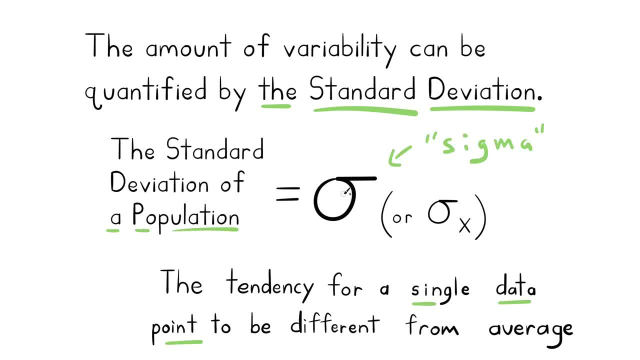 If our variable was height, this would be referring to the height of one person. Something like income has a higher standard deviation than height, because income varies a lot more than how tall people are. I mean, some people have billions of dollars. That's a huge amount of variation. 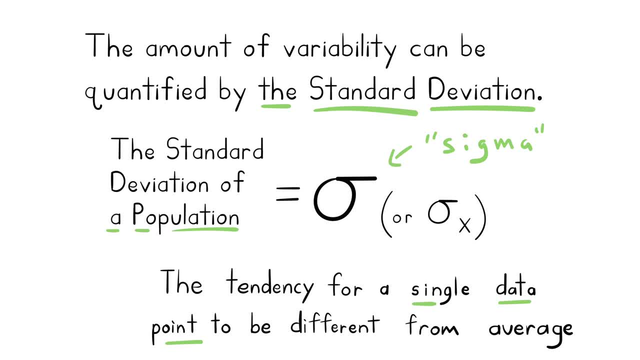 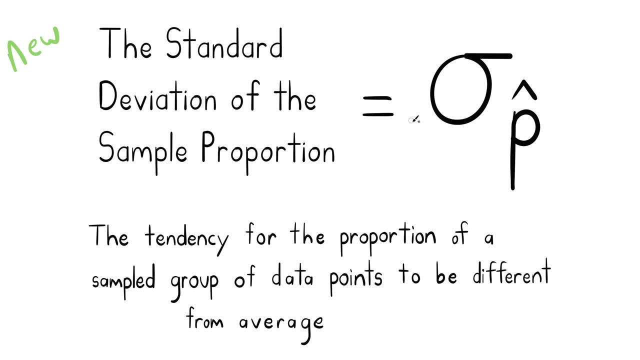 Nobody is billions of feet high. That would be a very tall person. Now we can talk about the standard deviation of the sample proportion, And that's going to be sigma, like we used before, but we're going to put a subscript p-hat on it. 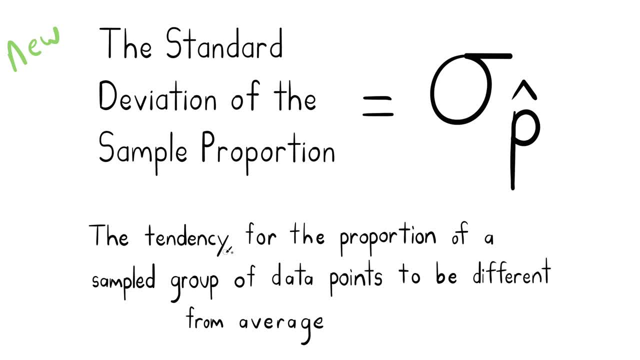 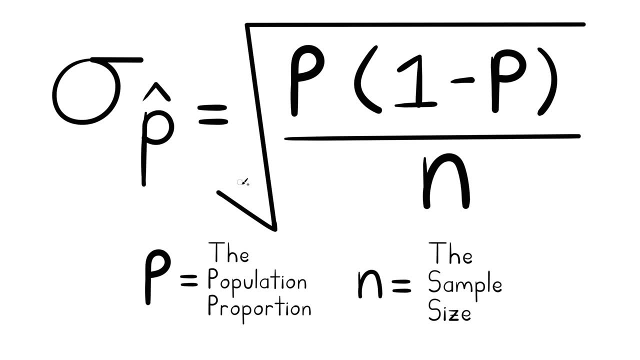 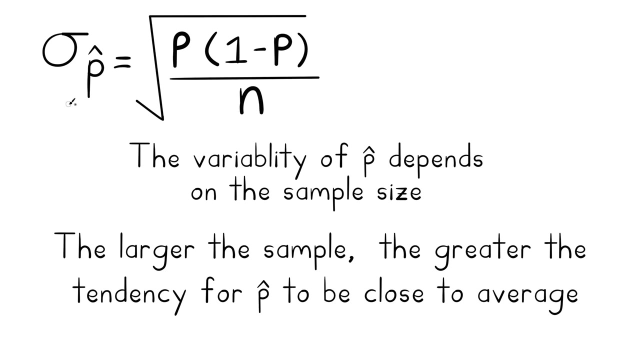 Sigma of p-hat is the tendency for the sample proportion to be different from average, And so this is a quantity, It has a formula, And what that formula looks like is where p is the population proportion and n is the sample size, And an important thing to notice is that the variability of the sample proportion depends 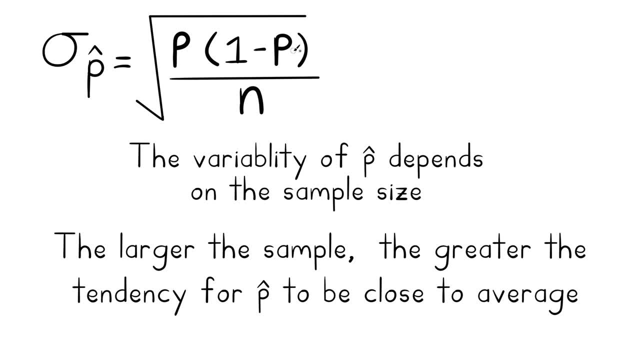 on the population proportion, because that's in this formula, But it also depends on the sample size. n. As a statistician, that's something that you potentially have control over. The population proportion is a characteristic of your population. that's not changeable. 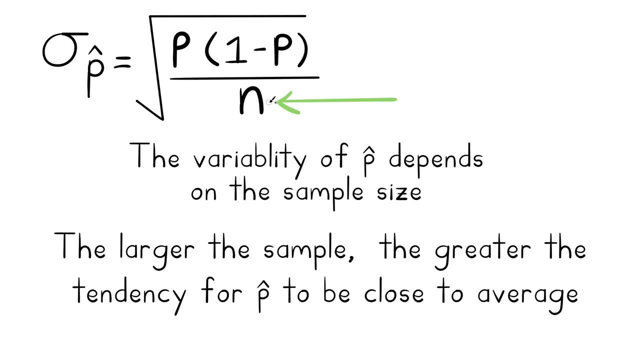 But the sample size is something that could potentially be changed, And this is a fraction with the sample size on the bottom, which means that if you have a larger sample, what happens with a fraction when the bottom gets bigger is that the entire fraction gets smaller. 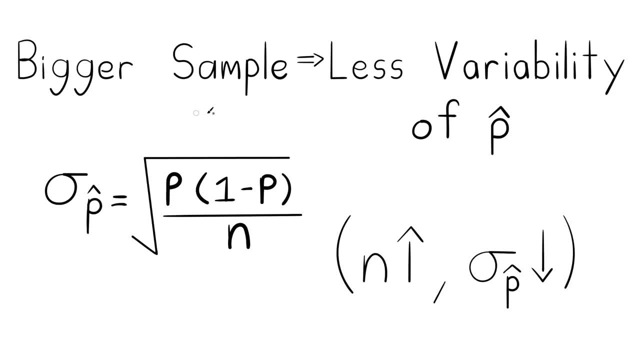 Let's look at that in another way. Let's look at that in another way. The bigger the sample, the less variability of p-hat, And that can be useful if you're trying to estimate a population proportion. The larger the sample you take, the greater the tendency for your sample proportion to 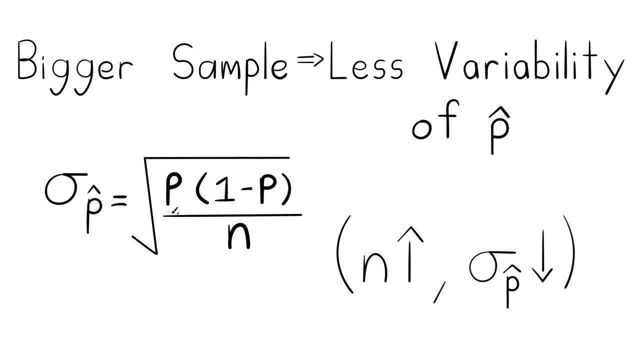 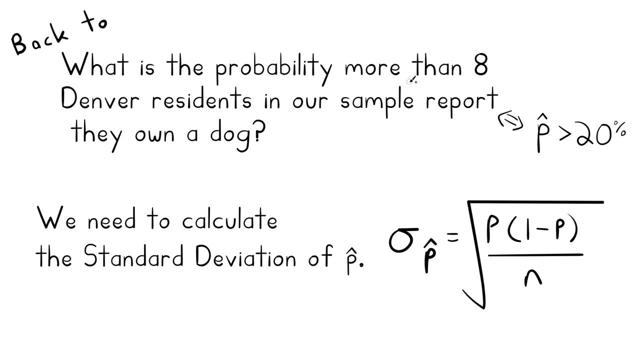 be close to the population proportion, which is a good thing. We're now ready to go back to our question of what's the probability that more than eight Denver residents in our sample report they own a dog. We're going to need to calculate the standard deviation of p-hat to find this area. 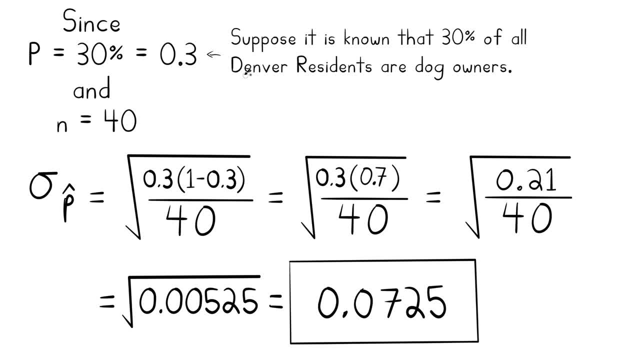 So okay, because we know that 30% of all Denver residents are dog owners, that's our p, That's 30%. We need to use the decimal equivalent of that. So here's our p times 1 minus p over our sample size. 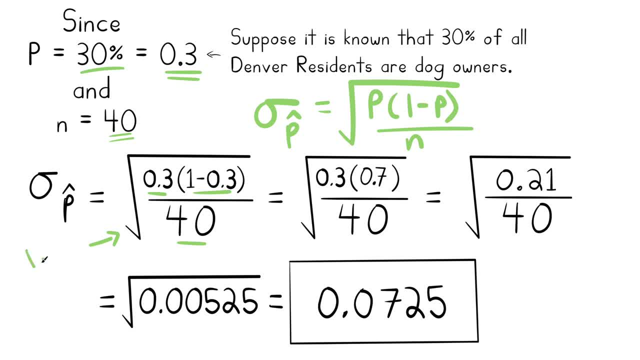 And eventually we're going to take the square root, but that's the very last thing we do. We'll do the subtraction first. That gives us 0.7.. 0.7.. We'll multiply these two numbers next. That gives us 0.21.. 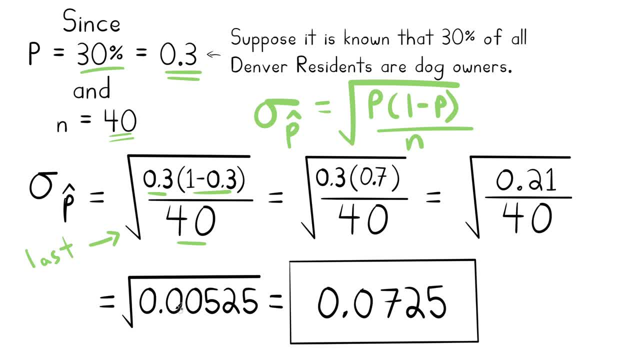 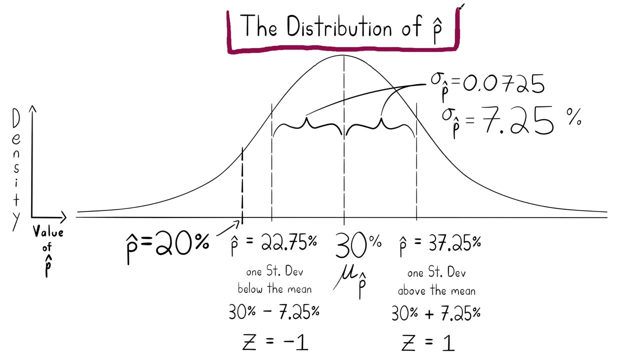 We'll divide by 40, next. That gives us 0.00525.. And then, lastly, we'll take the square root, which gives us 0.0725.. That is our standard deviation of the sample proportion, And so now we can have a more complete picture of what the distribution is. 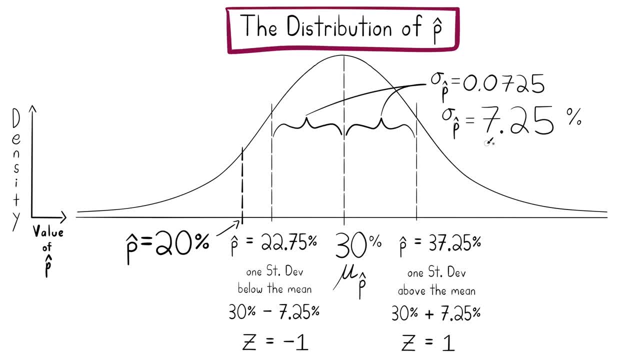 of p-hat looks like. Now we know the standard deviation, and so we could say things like: one standard deviation below the mean would be 22.75 percent, which means that the p-hat value that we're interested in right now is down here. It's further below the mean than just one standard. 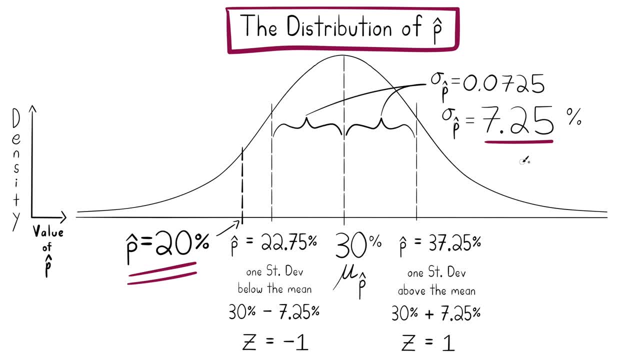 deviation. Finding the standard deviation of p-hat is the last piece of the puzzle. It's the last piece of information. we need to find any probability related to the sample proportion. Let's look at 20 percent and figure out exactly how far below the average it is. How many standard? 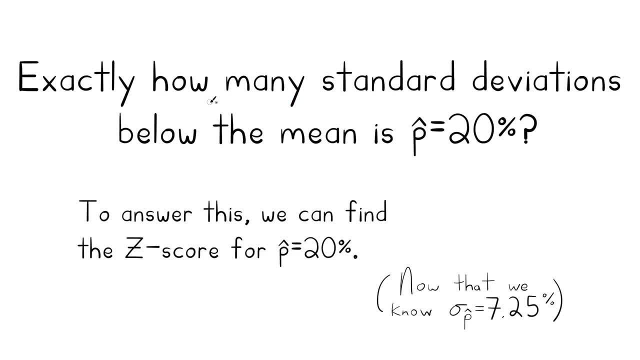 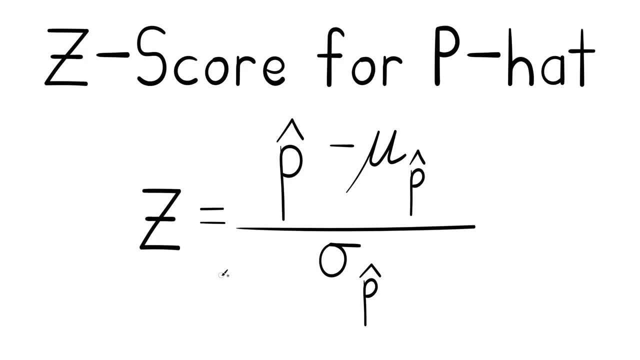 deviations, And so to know exactly how many standard deviations 20 percent is, we can find a z score. It turns out that if you ever want to find a z score for a value of the sample, you need to find the standard deviation of p-hat. So if you find a z score for a value of 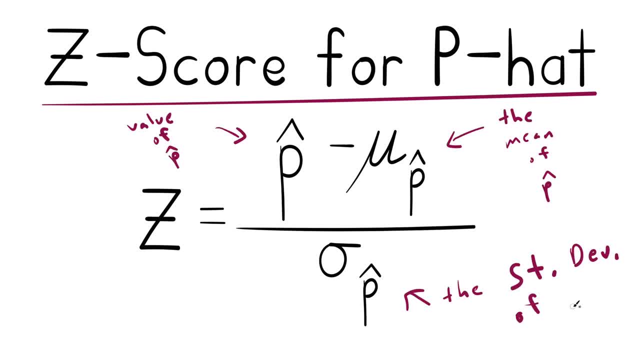 the sample, you need to find the standard deviation of p-hat. So if you find a z score for a value of the sample proportion, you can use a formula that looks like this, And this is actually the same format as any z score: We take the value of the variable, we subtract its mean and we divide by. 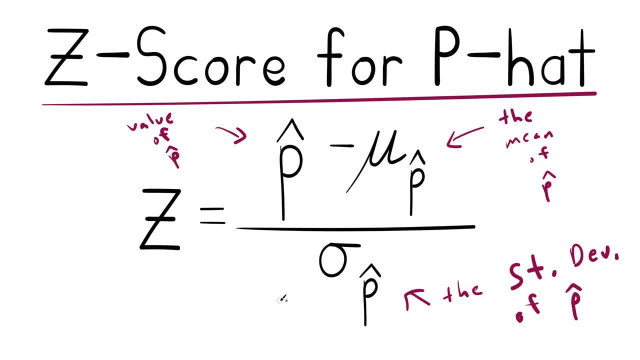 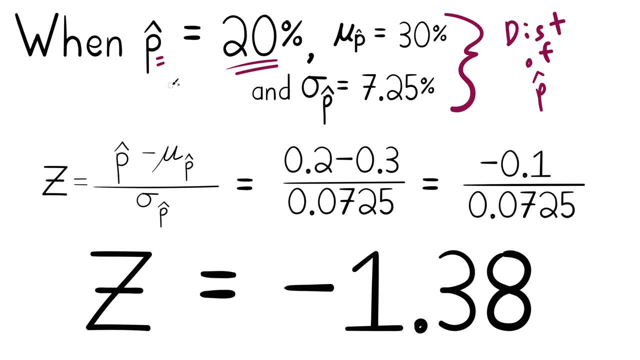 its standard deviation. This process is called normalizing it. So let's do that. So we had our p-hat value of 20 percent. So the z score is: take 20 percent as a decimal subtract 0.3, because that's 30 percent as a decimal divide by. 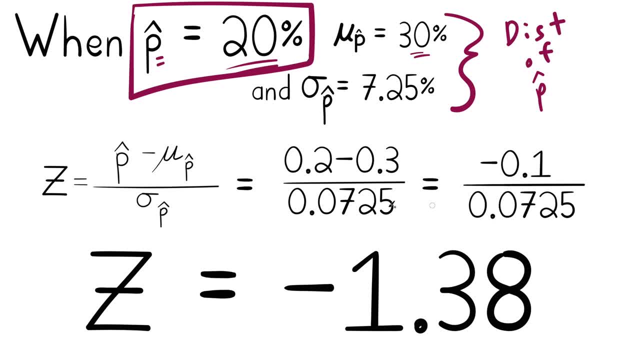 our standard deviation as a decimal, And when you do that, you get the z score for p-hat equals 20 percent. It's negative and it's negative 1.38.. What that tells us now is that our value of 20. 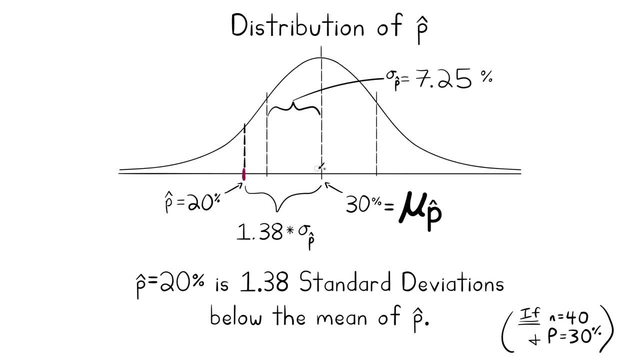 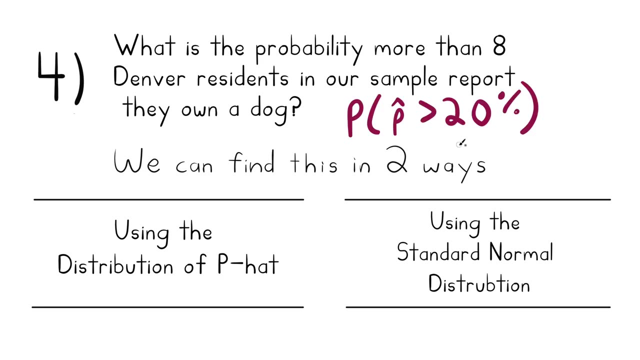 percent is exactly 1.38 standard deviations below the mean. The goal is to find this area here, but now we're getting closer to being able to do that, And it turns out that you can find this in two ways. You can just use the. 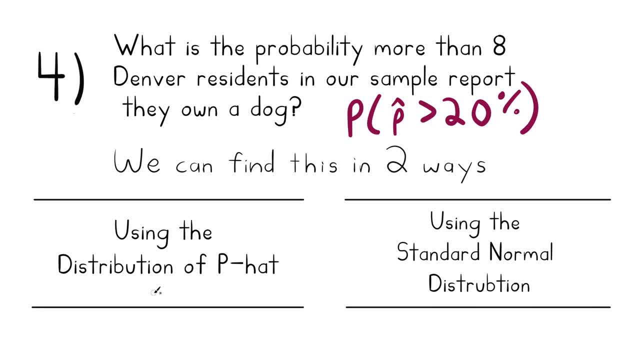 distribution of p-hat directly. This is my favorite way to do it, because typically this is a little bit less work. Or- and this is the method that a lot of textbooks do- they take any normally distributed variable and they turn it into a z score. It's really up to you. If it were me, I would just go ahead and do that. I would just go ahead and do that. If it were me, I would just go and do that. I would just go ahead and do that. I would just go ahead and do that, I would just go. 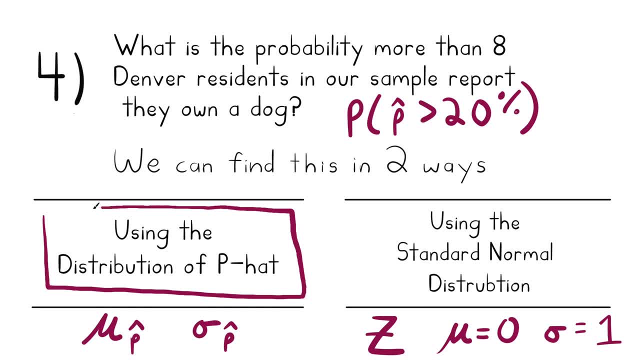 right to the distribution of p-hat, And this is assuming that you have a computer or a calculator or something that allows you to work with a normal distribution that has some specified mean and standard deviation. So let's just jump into what these two different methods look like. So if we're 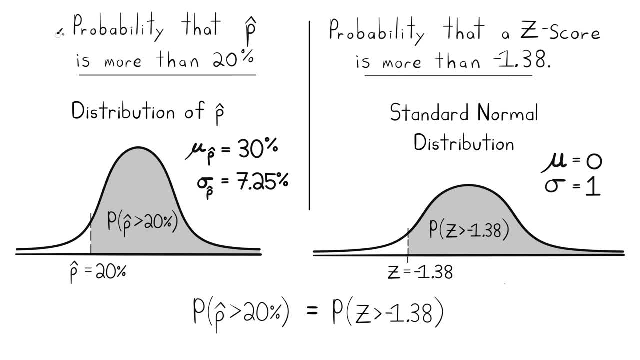 using the distribution of p-hat, we're trying to find the probability that p-hat is more than 20 percent. So we could find the area to the right of 20 percent Using this mean and this standard deviation, Or we could use the standard normal distribution. 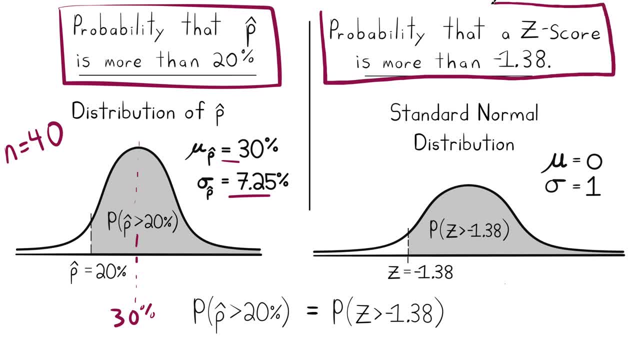 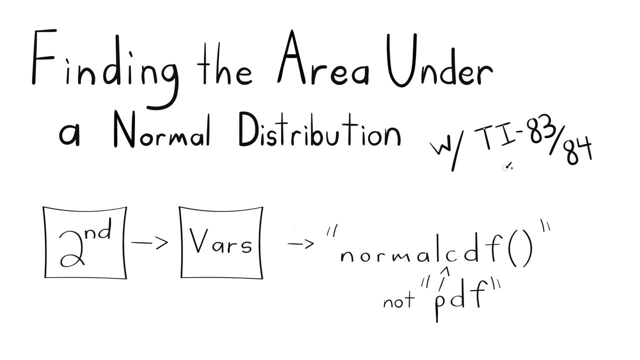 and find the probability that a z score is more than negative: 1.38.. And whichever one of these methods we want to use will get the same number. They're the same value. So you have a choice. And, as a quick reminder, there are many, many ways to find the area under a normal distribution. 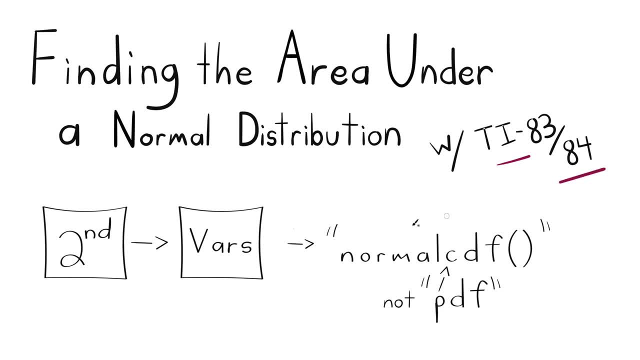 If you're using a TI-83 or a TI-85, you're going to have to find the area under a normal distribution. If you're using a TI-84, you hit the second button and then the button called VARS, And then you get a menu of. 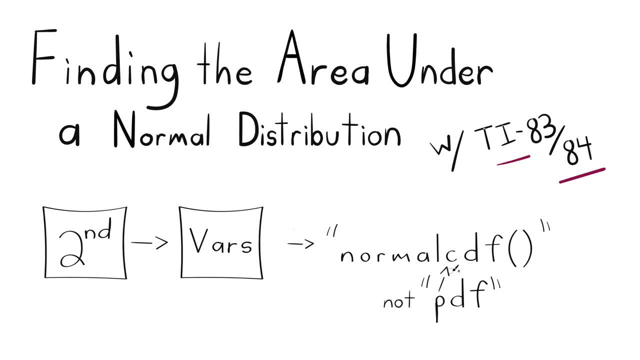 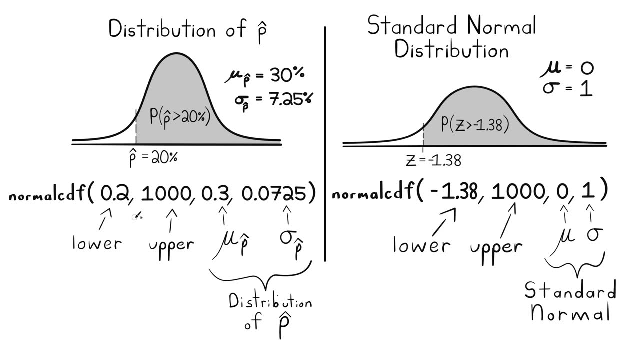 different items And we're looking for normal CDF, not PDF, Which, if you're curious, stands for cumulative density function. So here's what it looks like using normal CDF. This is exactly what you see in a TI-83.. A TI-84 looks slightly different, but you still need four numbers. 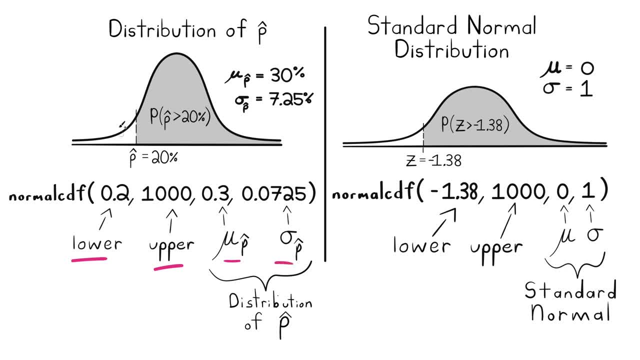 And the first two numbers are for the area that you want. So we're telling it to start here and to keep going for a very long time until we get to all the way to a thousand, which is crazy far. this way. You just need a big number here. You had to use 0.2 here because we needed to start there And 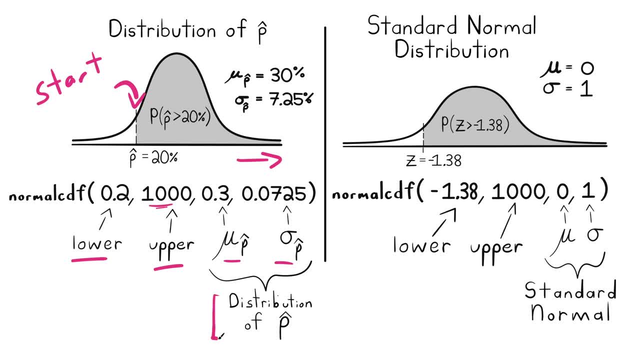 then the key here is that we're working with the distribution of p-hat. So we need to give the mean of p-hat as the third value And the standard deviation is going to be 0.2.. And the standard deviation of p-hat as the fourth value. And if you wanted to do this same sort of calculation, 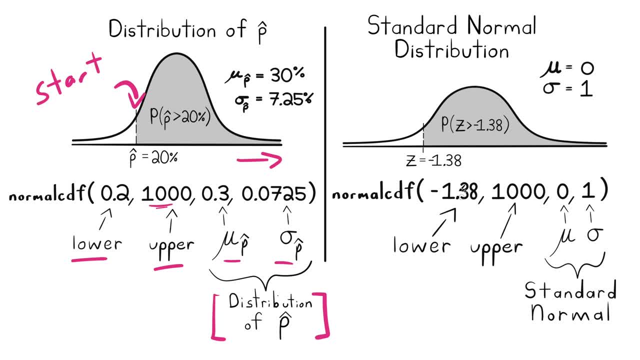 with a standard normal distribution, you would use your z-score as the start, And now we use the mean and the standard deviation of the standard normal distribution And obviously you wouldn't do both of these calculations. We're going to get the same number, My preferred method. 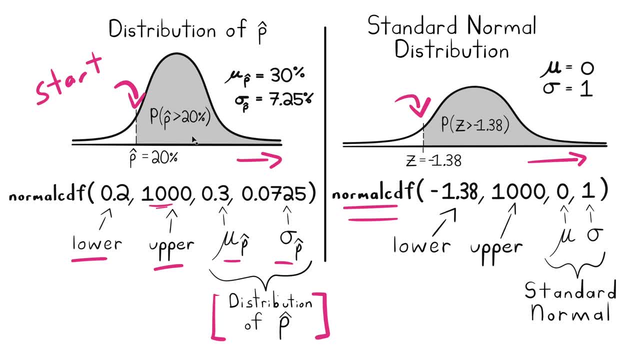 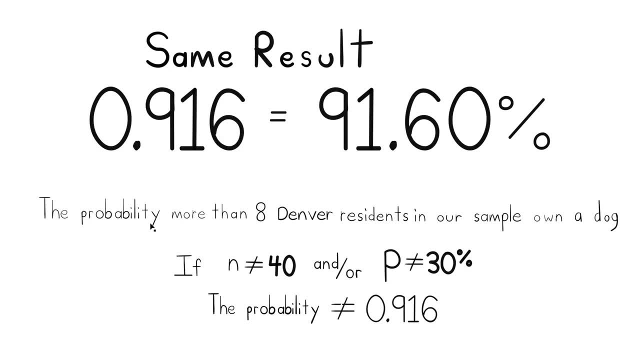 is the method on the left because it's a little bit quicker. I could have used this method without calculating a z-score And regardless we get the same result. We get 0.91691.6% because this 91.6% is the area to the right of 20% for the sampling distribution of p-hat, which is dependent. 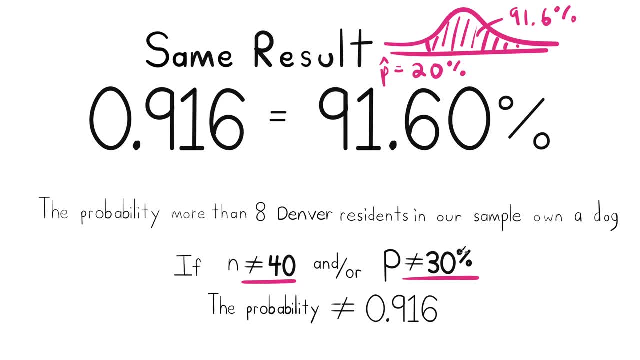 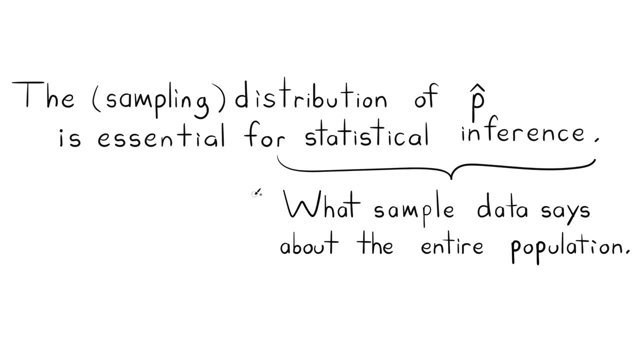 on the sample size and the population proportion. So if either one of those numbers changed, then the area to the right of 20% wouldn't be 91.6% anymore. So summarizing what's going on here. we just looked at the concept of the sampling distribution. 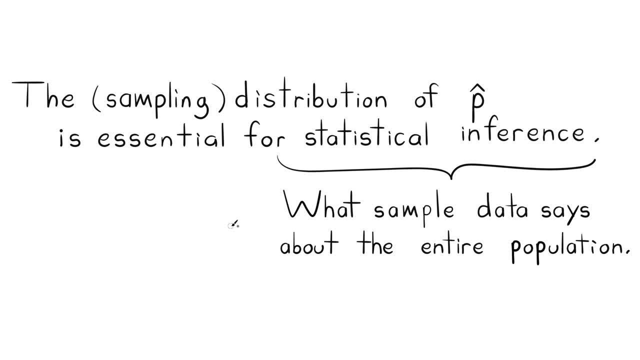 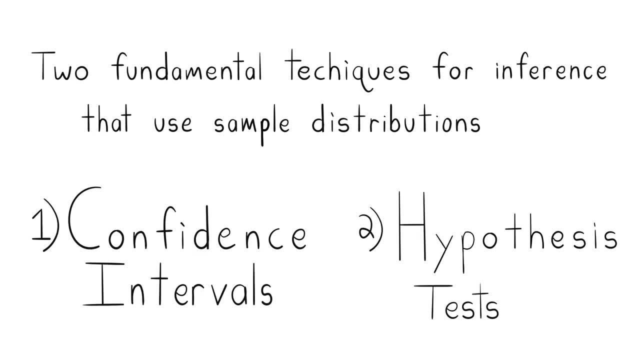 of p-hat. It's important for knowing what a sample says about the entire population, which is really one of the biggest themes of statistics, And it turns out that there's two main types of techniques in statistics that use sampling distributions, Confidence intervals. 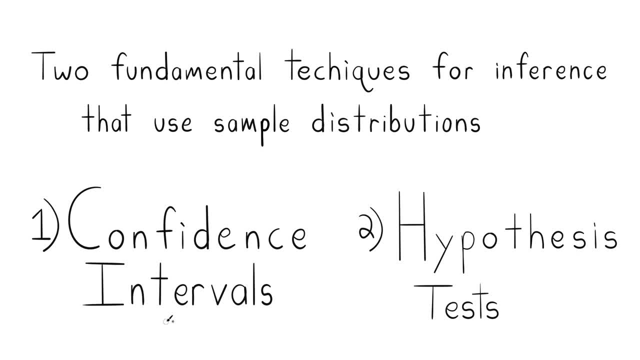 where you're trying to estimate the value of your parameter by using an interval instead of just one number. And the second one is called hypothesis tests or hypothesis testing, where you're trying to test some claim about a parameter. I have lots of videos on both confidence intervals and hypothesis. 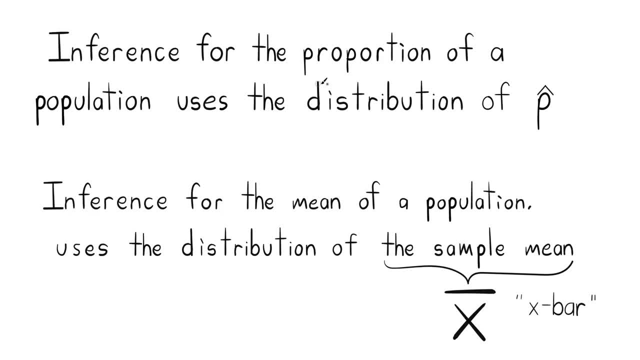 tests, And so if we wanted to make an inference for a population proportion, then we use the sampling distribution of p-hat. If we want to make inference, either estimating or testing a researcher's claim in a hypothesis test for a mean being mu, then we use a sampling distribution. But we'll use the sampling distribution. 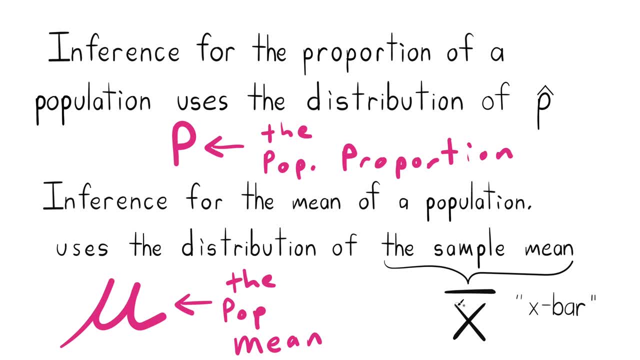 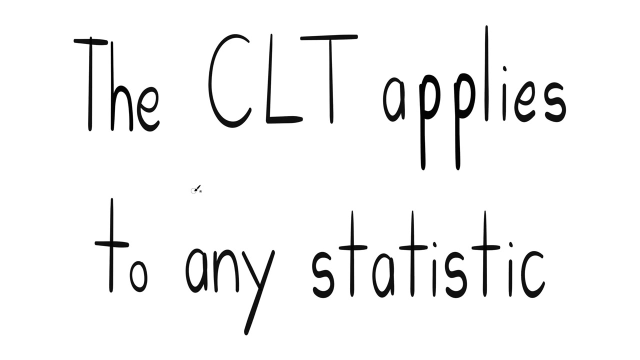 of the sample mean instead of x-bar, Basically just the idea that the sample mean varies, just like the sample proportion varies. So these are two statistics where sampling distributions are extremely useful to make inferences about their corresponding parameters. And one really cool thing is that the central limit theorem applies to any statistic. so a statistic. 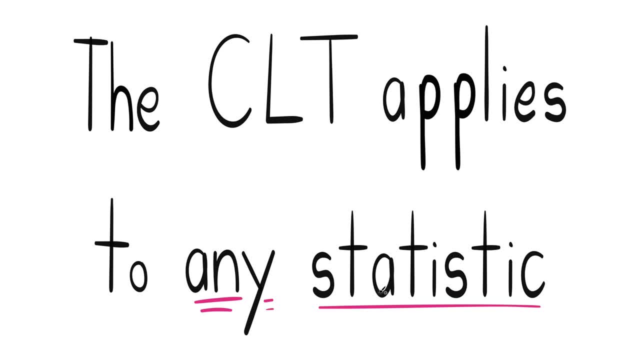 meaning a number that you calculate from a sample. If you calculate the same kind of number from multiple samples, the central limit theorem tells you that, whether that's a mean or a proportion or even something like a standard deviation, that statistic is a mean. 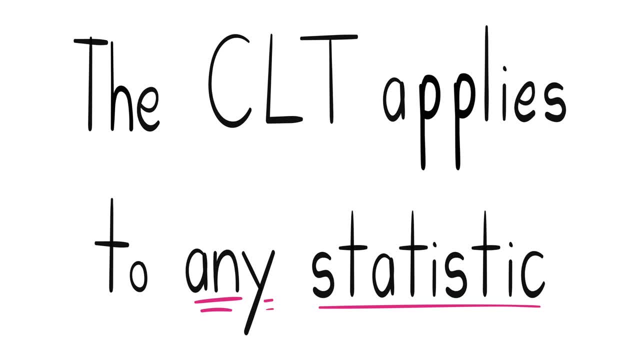 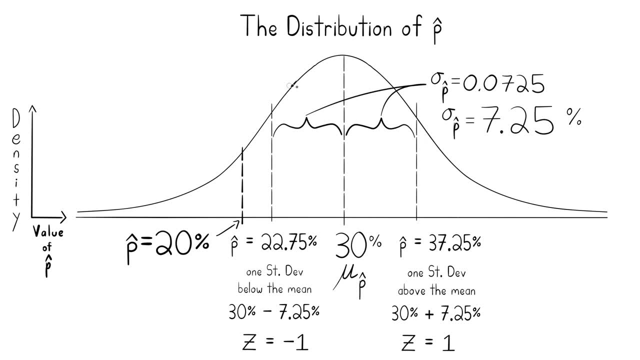 will be normal, will be bell-shaped, which is really cool, I think. So, summarizing what we've learned, we've talked about the sampling distribution of p-hat, which has a normal shape. if your sample size is big enough, your population is big enough compared to your sample and your 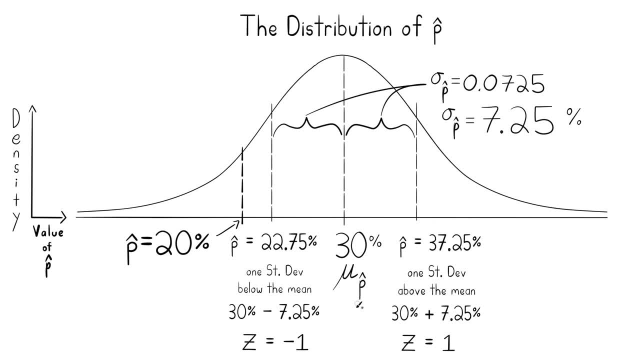 sample is taken randomly and that distribution has a middle, which we can call mu of p-hat, and mu of p-hat is just whatever the population proportion is, and that normal distribution has a standard deviation which we call sigma of p-hat. One of the really important ideas that 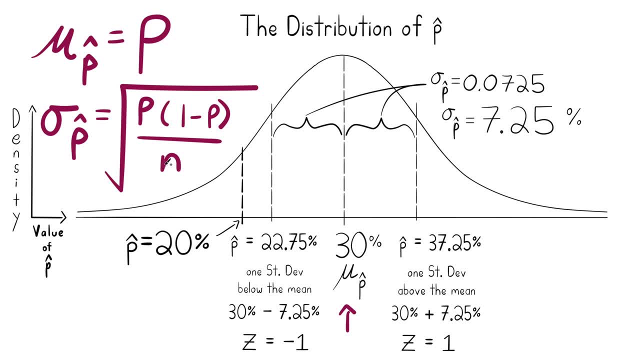 comes up here is that as the sample size increases, the standard deviation decreases. A larger sample ends up with this curve being more peaked in the middle, And a smaller sample gives you a curve that's more squished, flat, has more area on the outsides.